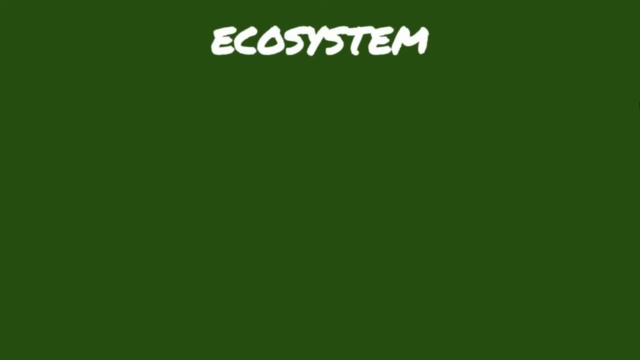 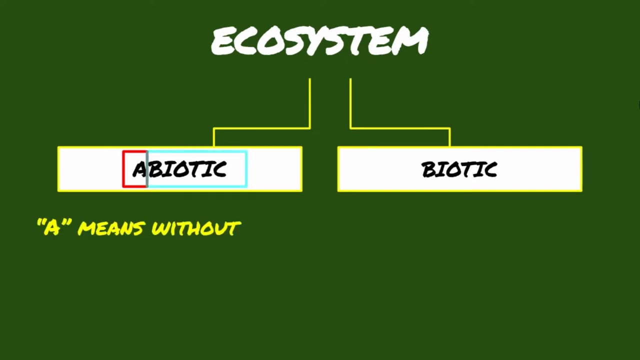 An ecosystem is made up of abiotic and biotic components that work together to maintain balance, preceded by the prefix a- which means without, followed by the Greek word bios, which means life. Abiotic therefore means without life, It is the non-living components. 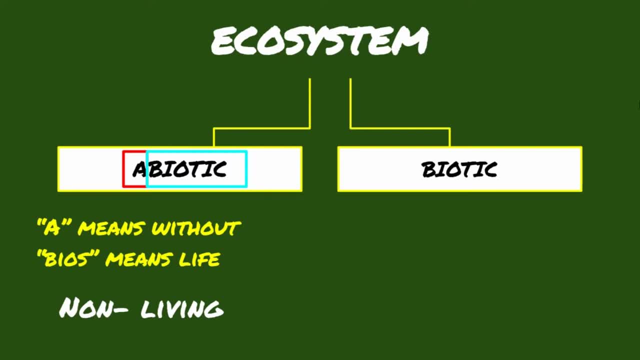 or the physical and chemical aspects of an ecosystem. On the other hand, the biotic component is the living component of an ecosystem. This includes all living organisms that are dependent to one another. This means that each living organism has a relationship to other living organisms. 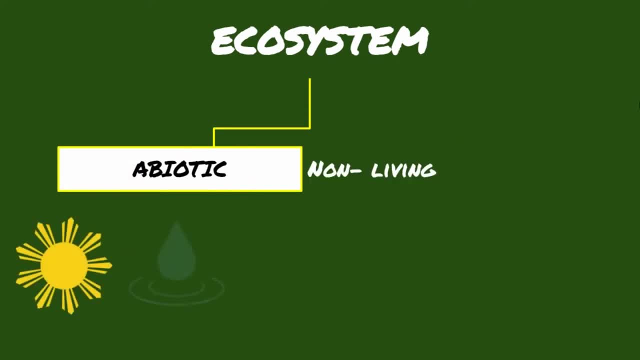 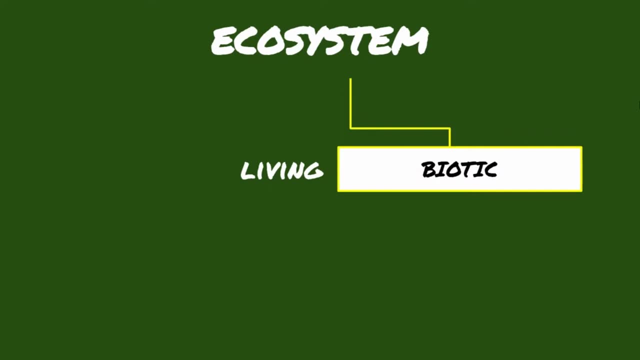 Abiotic components include the sun, water, air, weather, rocks and soil. Biotic components include various plants, animals and bacteria that act as producers, consumer or decomposers. Now let's differentiate both abiotic and biotic components in an ecosystem. 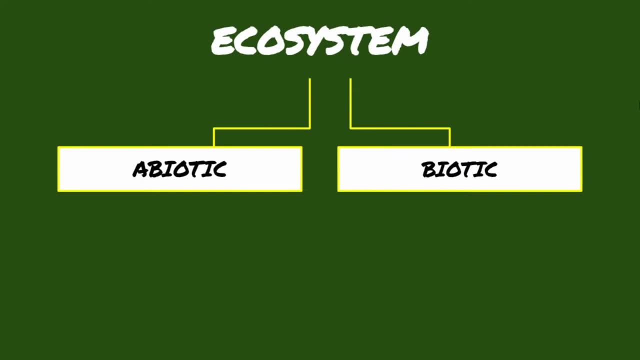 Abiotic components do not depend on biotic factors for their existence. With or without the biotic components, there will still be abiotic components in the ecosystem. On the other hand, biotic components depend on abiotic factors for their survival and growth. 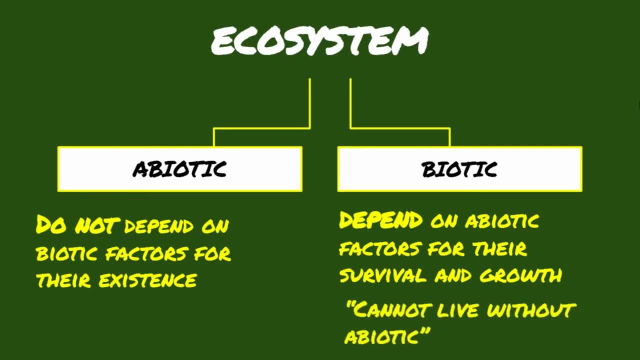 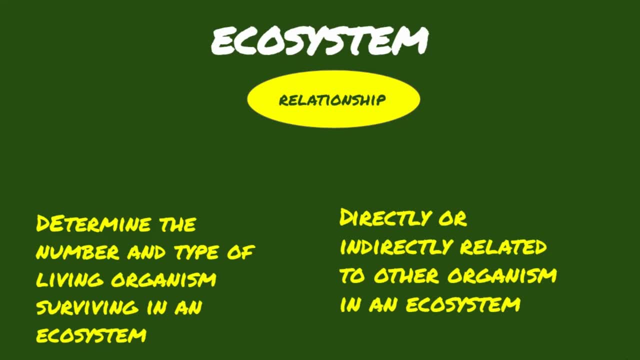 Meaning biotic components cannot live without the abiotic factors. In terms of relationship, abiotic factors determine the number and type of living organisms surviving an ecosystem. On the other hand, living organisms might be directly or indirectly related to other organisms in an ecosystem. 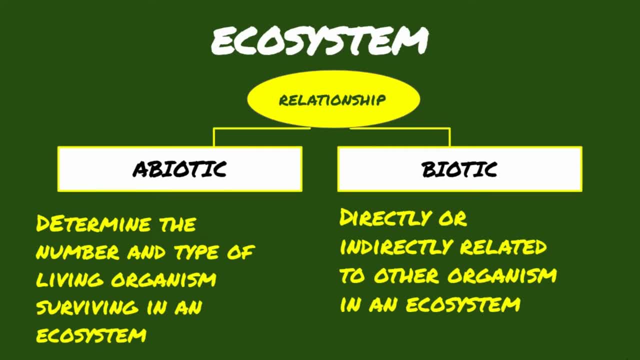 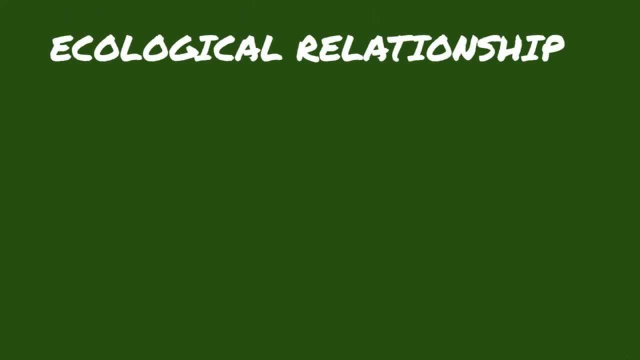 Interactions and relationships exist in an ecosystem in search for food, shelter and protection. These interactions may have positive, neutral or even negative influences on the interacting population. Some interactions are beneficial, while other are harmful. harmful: There are also interactions where population of organisms are neither benefited. 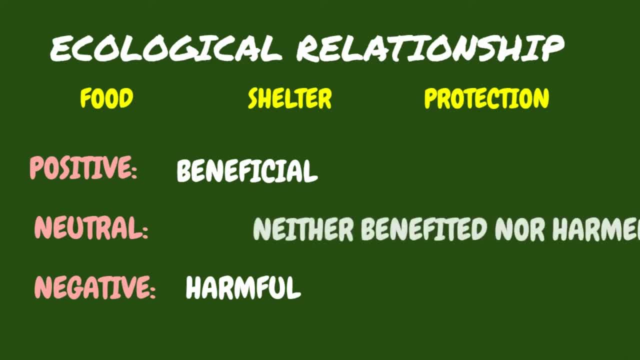 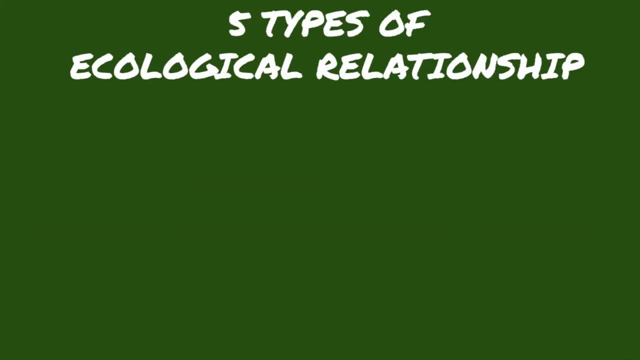 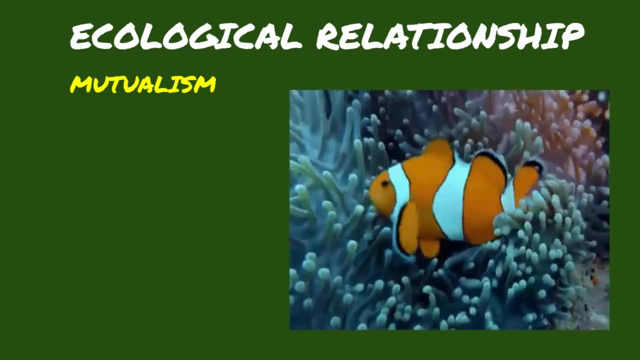 nor harmed. These interactions are called the ecological relationships. There are five types of relationships that exist in an ecosystem, namely mutualism, commensalism, parasitism, predation and competition. Let's start first with mutualism. Mutualism. 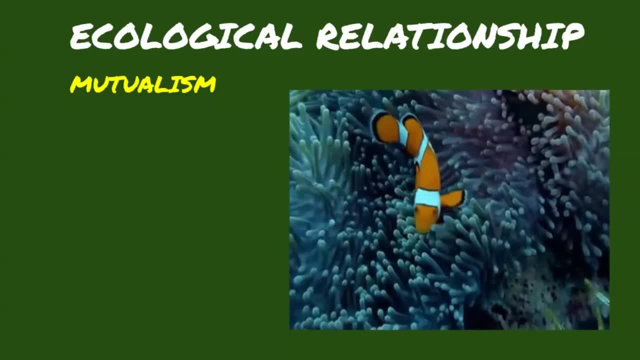 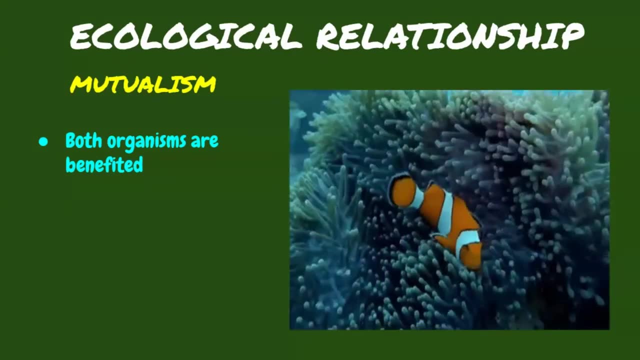 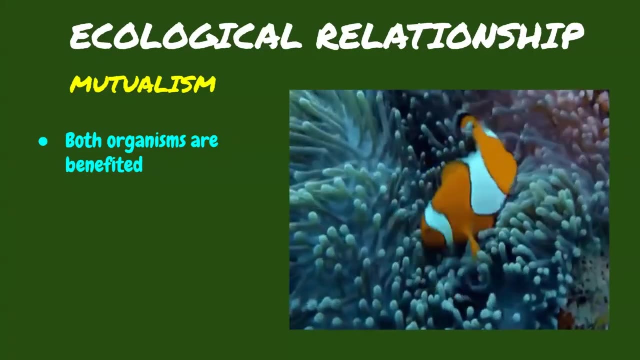 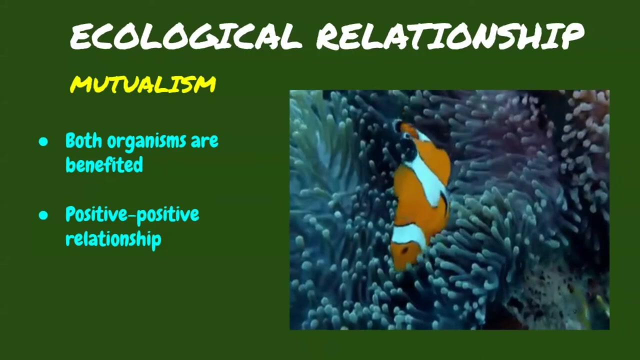 is an ecological relationship where both organisms are benefited. It plays an important role in the growth, reproduction and survival of the organisms and in maintaining the balance of the ecosystem. It exhibits a positive-positive relationship. Thank you. An example of this is the relationship that exists between clownfish and sea anemones. 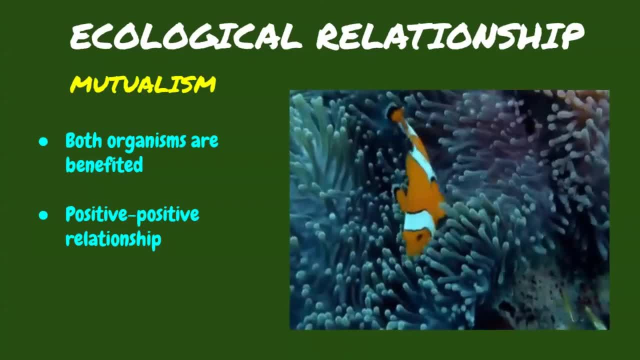 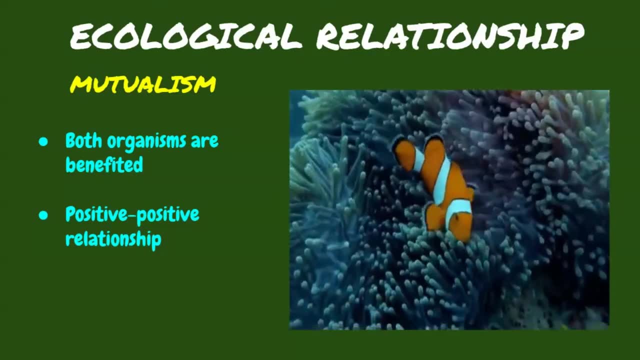 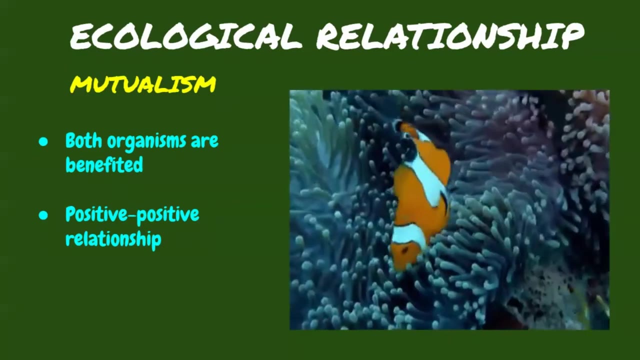 The clownfish provide the sea anemone nutrients in the form of waste, while also scaring off potential predator fish. while the sea anemone provides the clownfish rib protection and shelter, A remora fish would attach itself to a shark and use the shark as a bait to 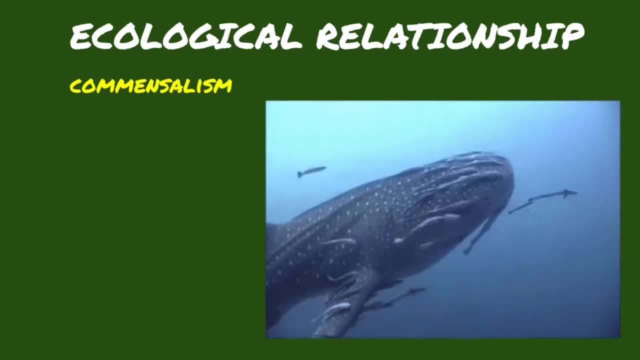 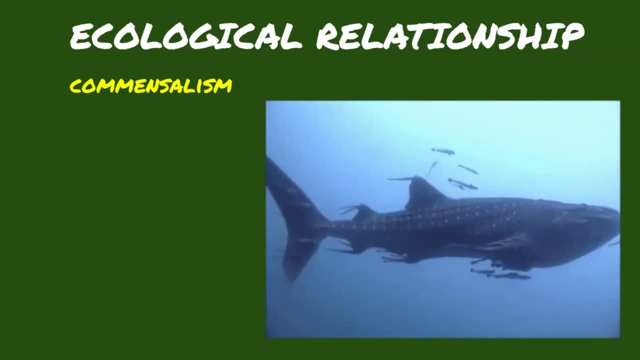 the shared domain to collaborate with to gum, conte and find the shark. Then the remora fish is feed the shark and, inseparable, The remora fish eats all the food that is left over from the shark. The symbiotic relationship between them is called commensalism, where 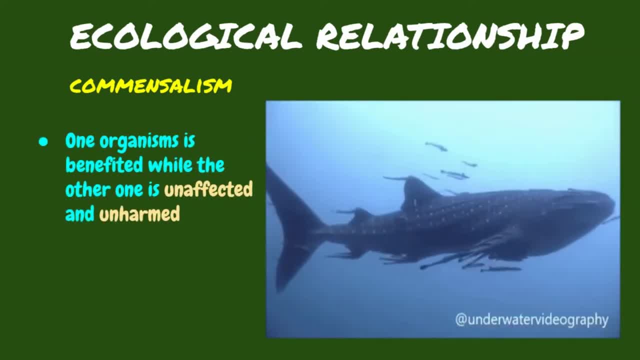 one organism is benefitted, while the other one is not affected nor harmed. The remora fish is getting its food, but the shark gets no benefit. This relationship usually exists between an organism and an earth. thereforeoke it deals more with power than strength. The 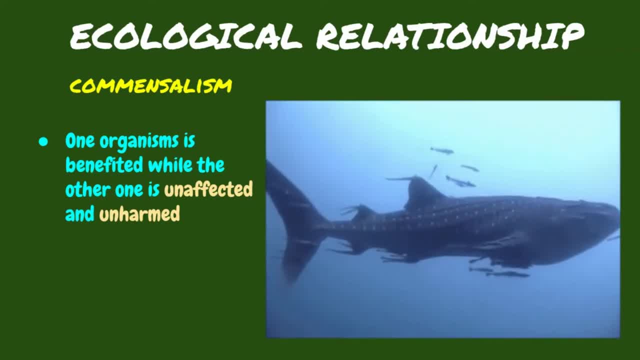 remora fish don't keep their own food but its Huang Lei confection After so lasting. in the smaller one, the organism which gets the benefits, it's called the commensal. the commensal uses the other organism or the host for transport, shelter or protection. this is a positive, neutral. 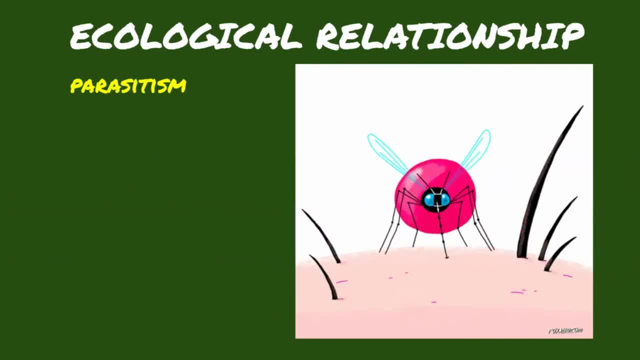 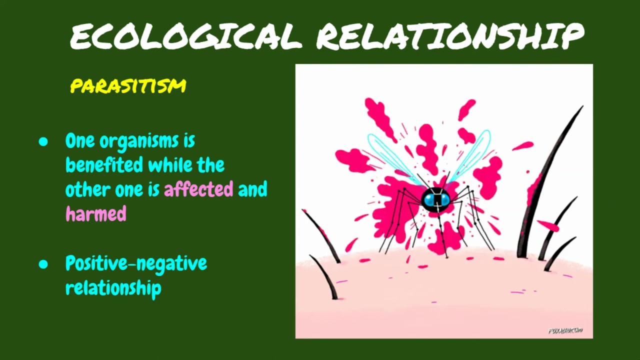 relationship. parasitism is positive, negative relationship, where one organism is benefited while the other one is affected and harmed. the organism that benefits from the relationship is called the parasites, which is usually smaller than the other organism, or the host. the mosquito is a parasite that lives outside the body of the host. it sucks blood from the skin of. 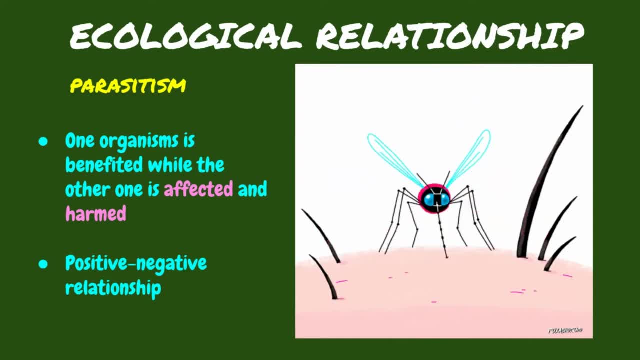 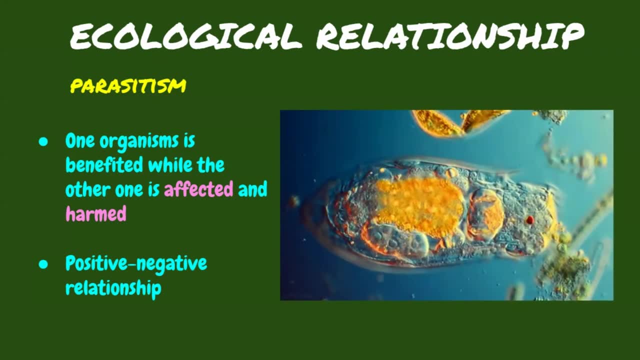 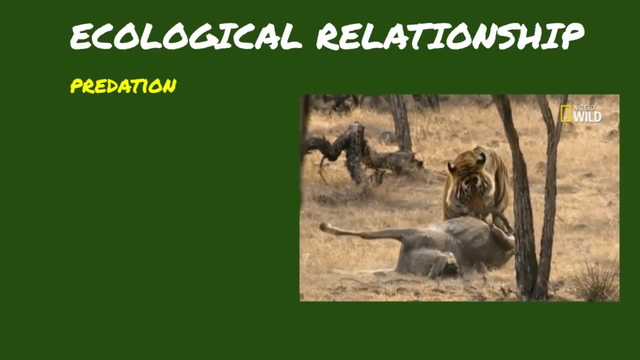 animals or humans, which are the host. there are some parasites that can cause diseases. bacteria and other microscopic organisms live inside the body of the host and cause diseases like pneumonia and malaria. another relationship that exists in the ecosystem is the food getting relationship. one organism is benefited while the other one is killed and eaten by the. 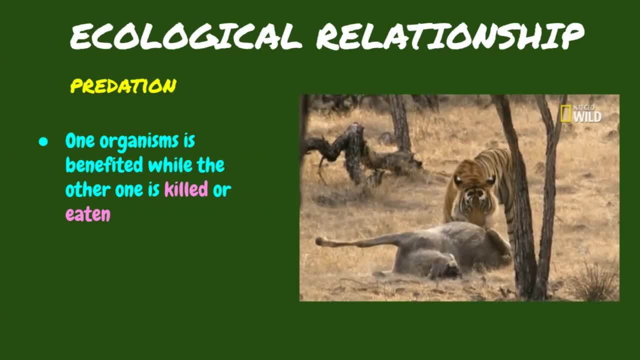 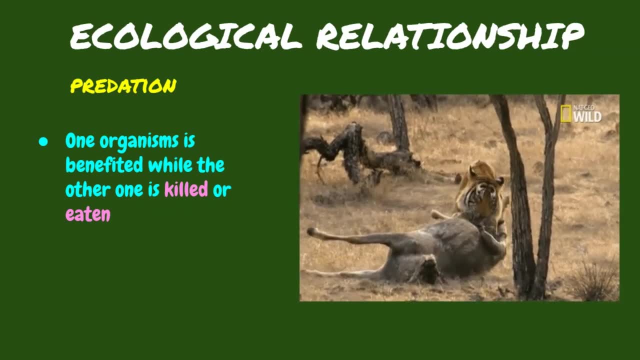 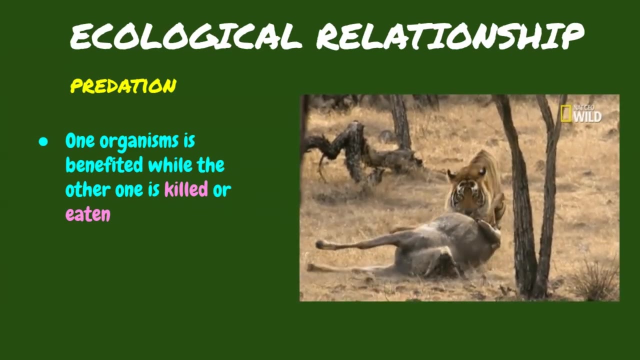 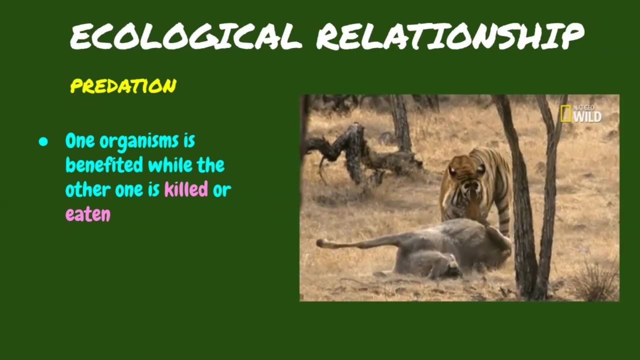 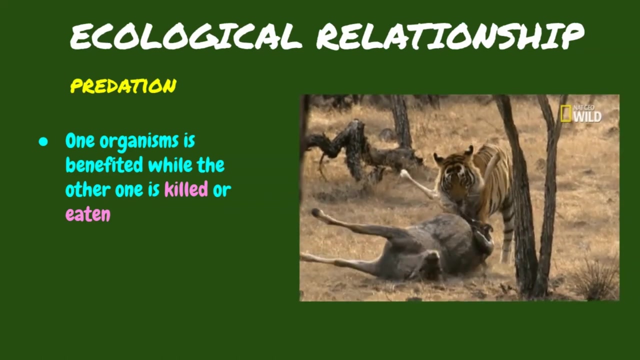 other organisms. this relationship is called predation. an animal that kills and eat other animals is called the predator. an animal that is killed and eaten by its predator is called the prey. the prey are less powerful than the predator that eats them. in a given community, predators compete with other predator for prey in the wild. a. 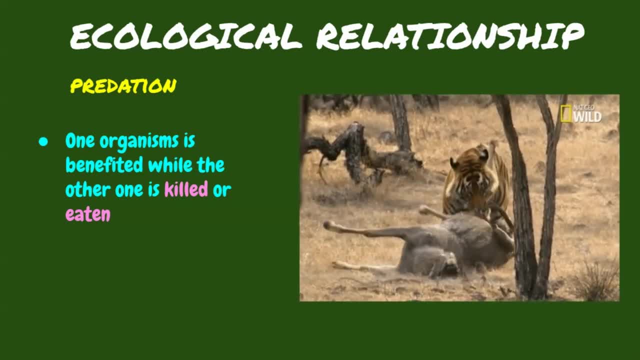 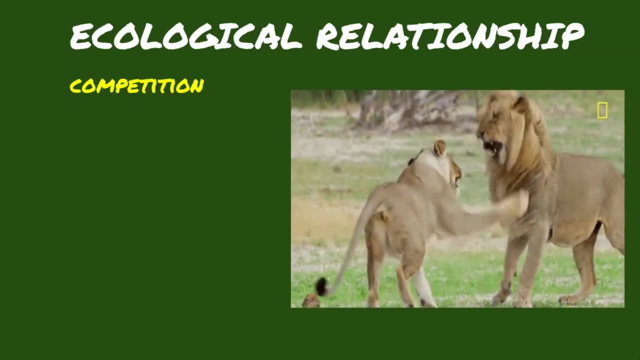 predator may be another prey of another predator that doesn't exist, an animal that kills and eat an predator. this means that while an animal haunts and feeds upon another animal, it can also become prey to a larger and stronger predator. in the ecosystem, competition takes place when organism 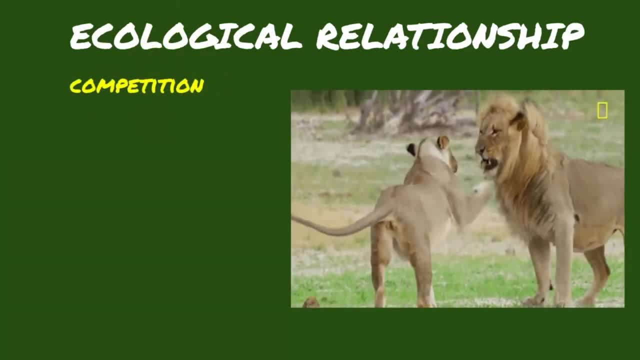 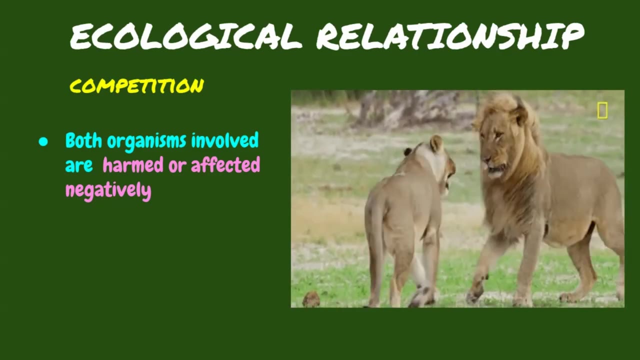 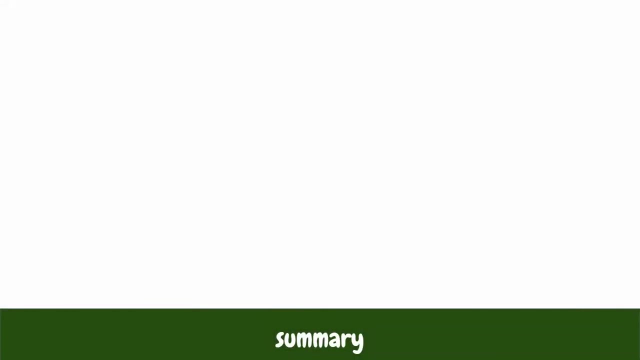 compete for limited resources like food, space, shelter or territory and mates. competition may happen between organisms of the same species or between different species. in competition, both the organisms involved are harmed or affected negatively. it has negative, negative effect on the organism. now let's summarize what we have learned today. an ecosystem is made up of